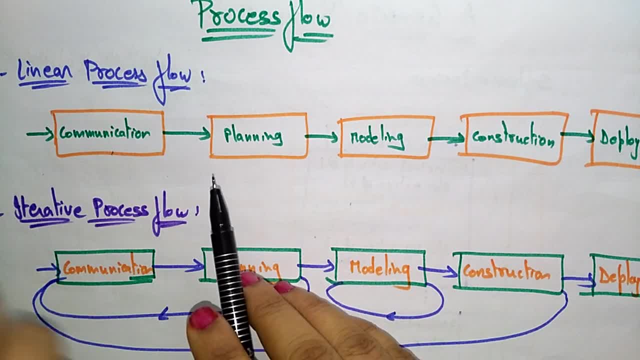 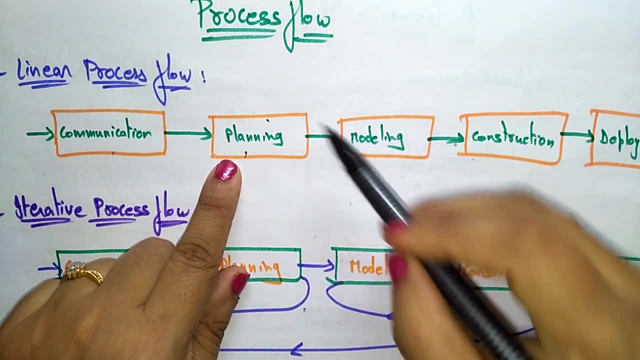 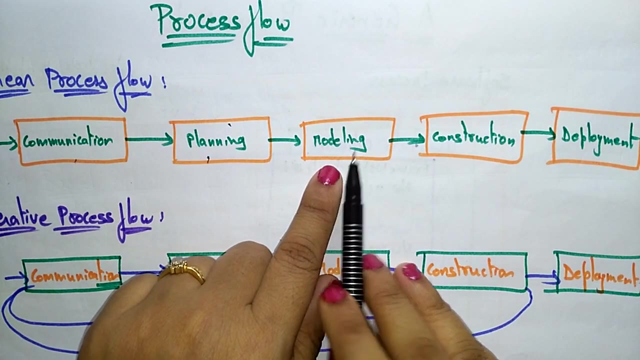 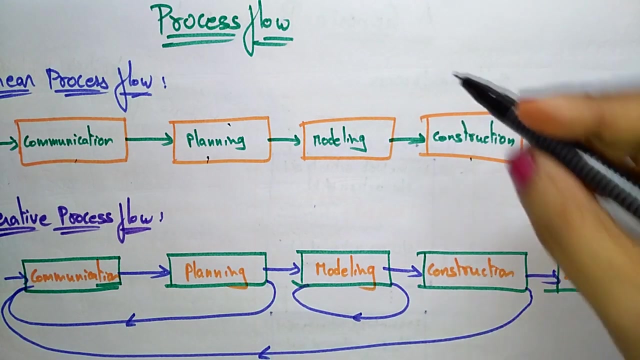 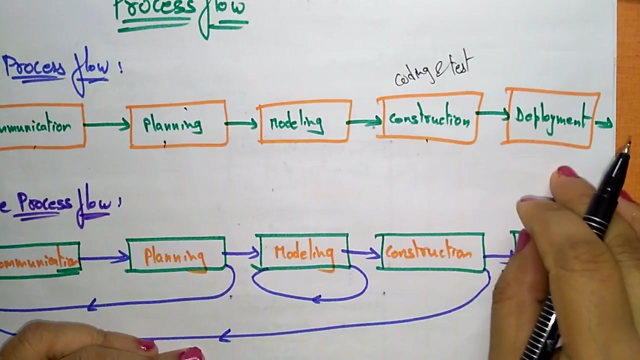 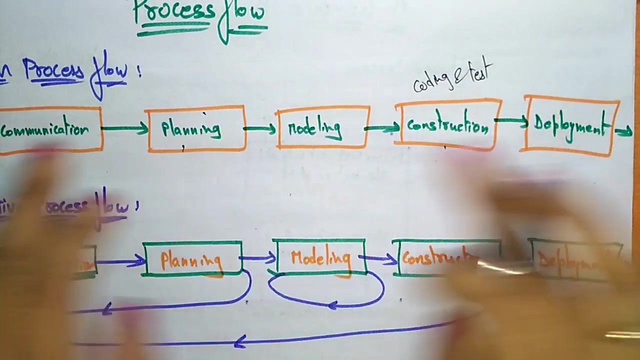 Okay, we are taking the developer has taken all the requirements and specifications from the customer, So then he is going to do a planning. After the completion of planning they can enter into the modeling. They are going to design the planning section After modeling by seeing the pictorial representation. the developer is going to construct the product Means their code and coding and testing is done in here- Coding and test. So after construction they have to deliver the project, That is, the deployment, or deliver the product Deployment. So this is a linear process flow going in a sequential way. So this is a one process flow. 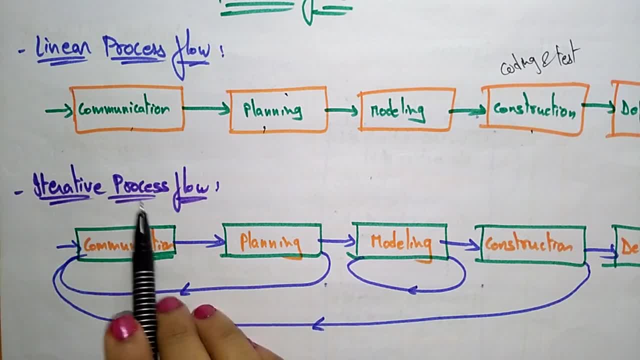 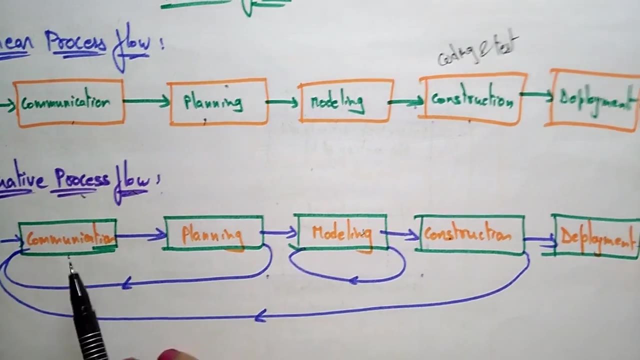 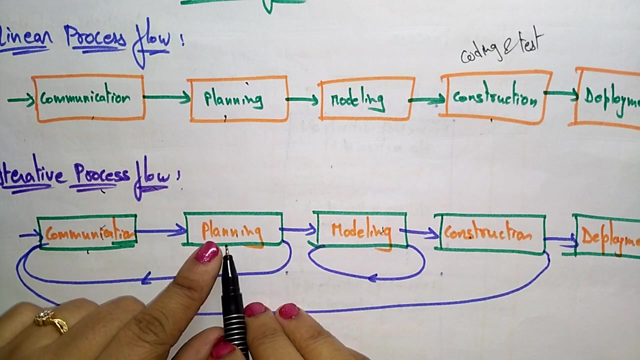 process model. now coming to the second type of process model, that is, a iterative process flow. iterative saying that is a loop condition, means continuously rotating like that. so the same faces communication, planning, modeling, construction and deployment. so once if the customer is communicated with the developer, if we take in some specification from the customer, the developer is going to plan. 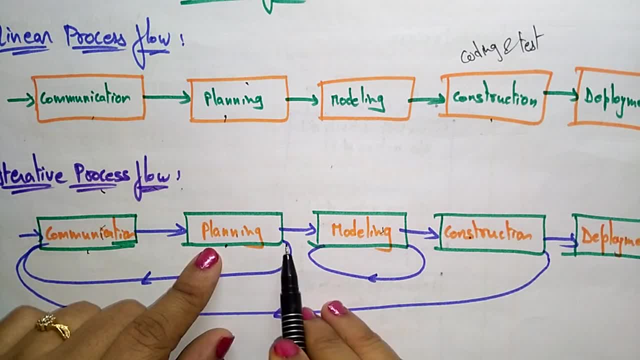 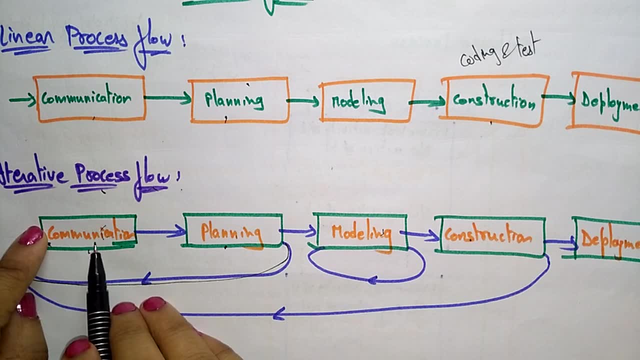 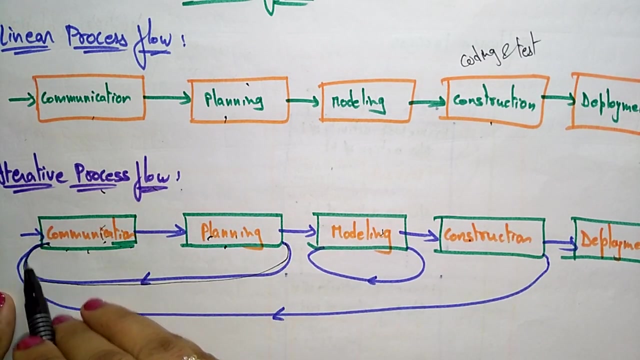 the project. so if we come some any doubts again he inquire the customer. suppose if the customer want to add some few points to that product, whatever he want, he just again communicate with the developer again. try to planning means this is a iterative process between the customer and 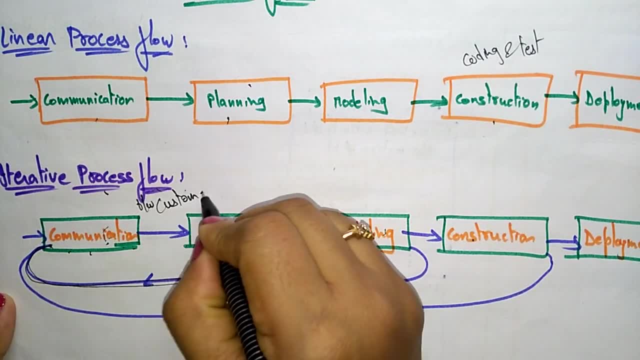 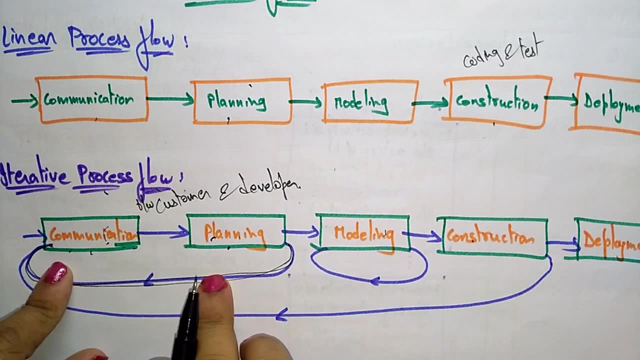 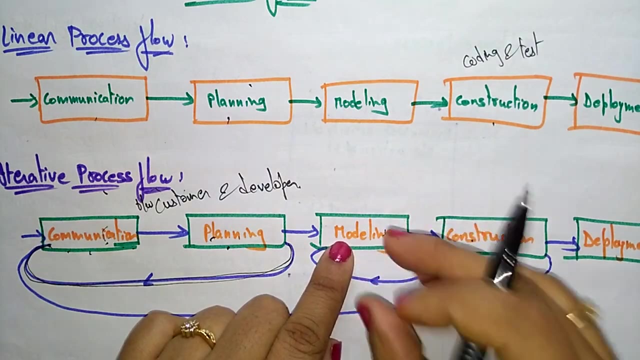 iterative process between the customer and the project. so if we come some any doubts again, he inquire the customer. suppose if the customer and developer- so that's why we call it as iterative process flow- okay, once a final, once final. they are doing the modeling, the developers are going to do the modeling, so they are not to freeze. 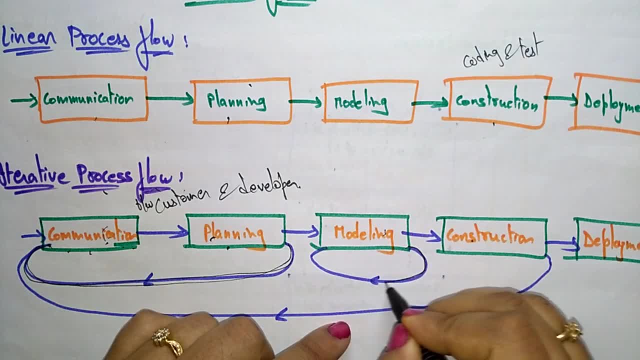 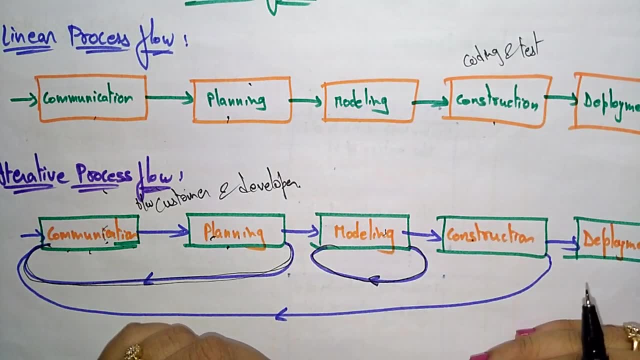 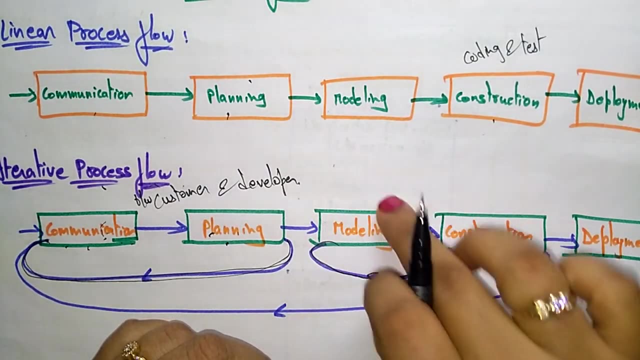 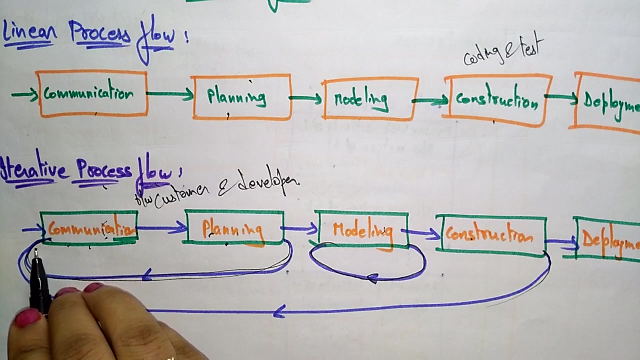 with only one task. they are always trying different, different ways. that is a modeling iterative. once they designed one model so they are still elaborating that modeling to some easiest means adding that enhance features. so this is the iterative process flow after construction. also, they again communicating with the customer before deploying the project. they are asking: is there any? 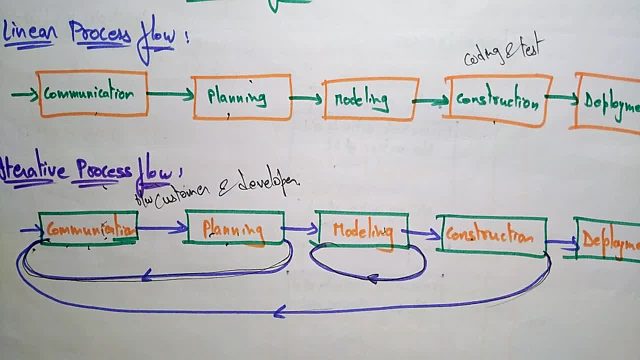 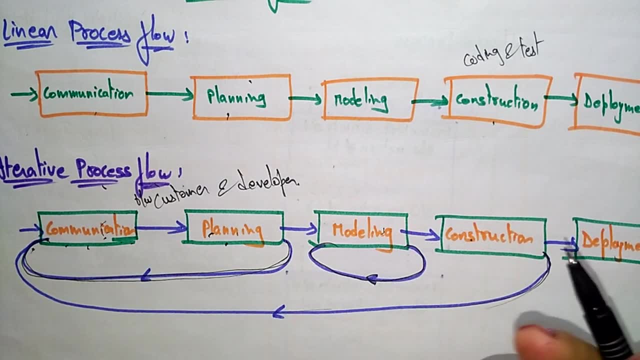 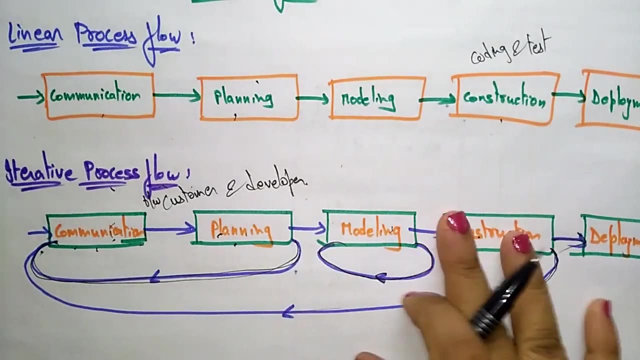 changes we have today, just like a prototyping, or just like it is in a spiral model, just after the construction. also, they are going to communicate with the customer. if there is still any enhancements will be there. so finally, they deploy the project, they deliver the project. so this is a iterative process, flow in each phase and iterations will be. 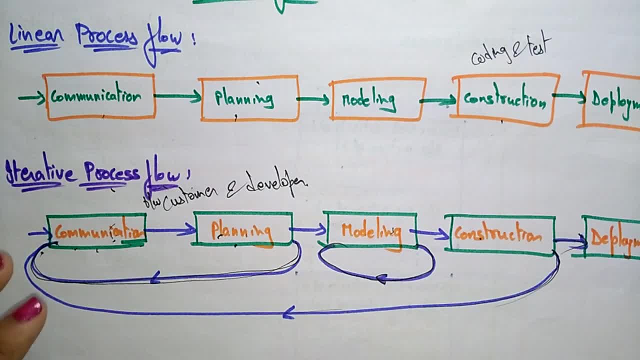 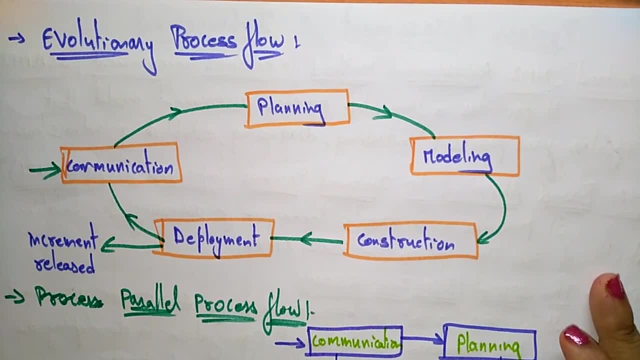 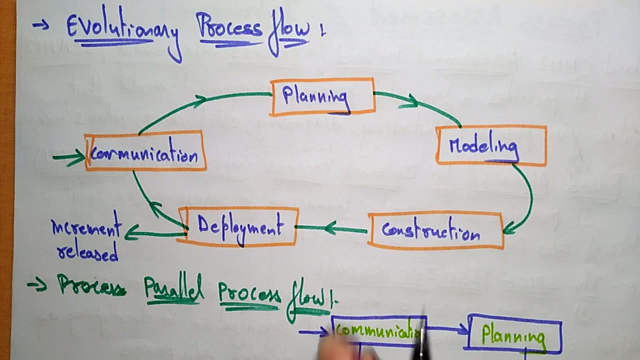 there in one or two phases, iterations will be going on. so the next, coming to the next process flow, that is a evolution, evolutionary process flow. what do you mean by this evolutionary process flow? evaluating the each and every phase? so once, if the customer and the developer is communication. 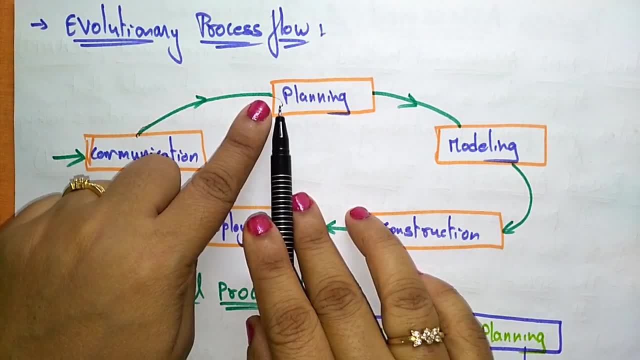 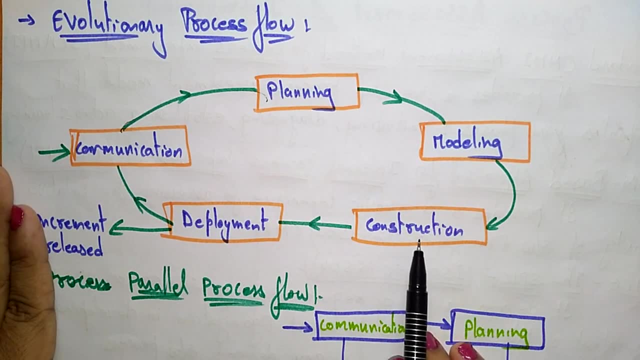 communicated, then they are starting the development, is starting the planning, the project. after planning, the documentation, everything is over. they are going to be modeled the project. after that they try to construct the project by writing the coding. after doing the coding, they are going to test the project. once that they are going to deploy the project. so 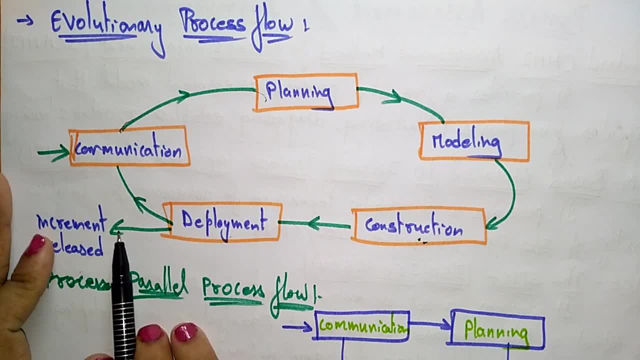 deployment will be given to the means the product is delivered to the customers. so, even though you develop, deliver the customers. they are going. the customer is going to be enhanced. the add the more features to that product. so this becomes the increment released. increment. again, they will be communicated. again, they will do all the if they. 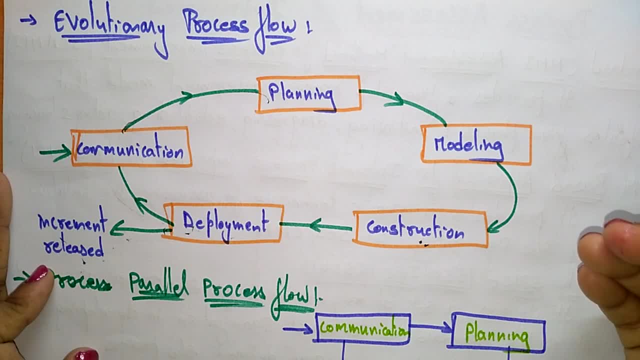 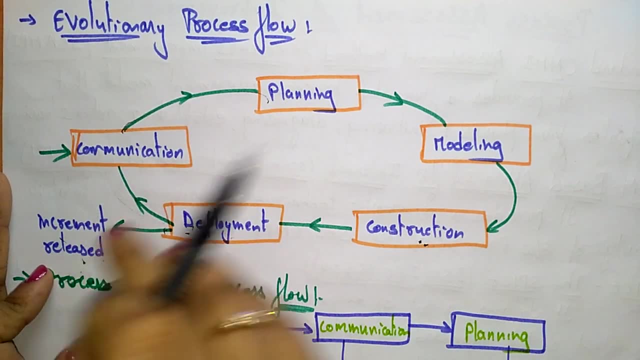 want to add some more module, if they want to add some more services to the pro project, means like that, the modifications will be taking place and again it will be released. this is an increment release. you call it as an evolutionary process flow. now coming to the next process flow, that is a 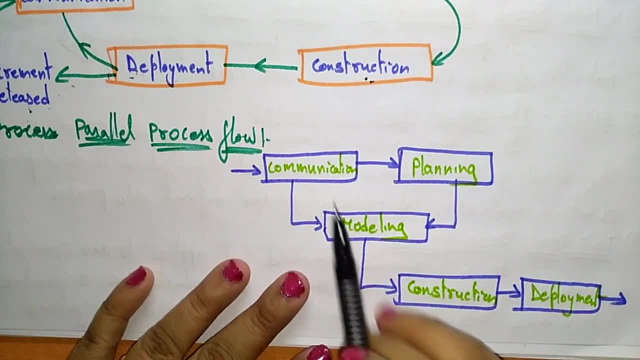 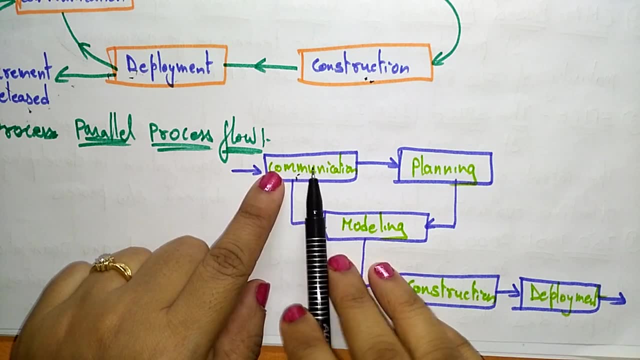 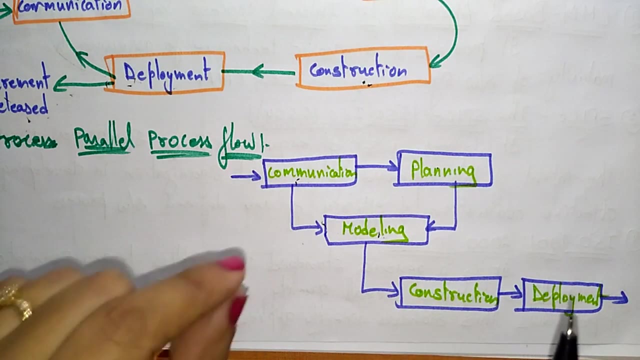 parallel process flow. parallel process flow: here communication will be taking place between the customer and the developer. so once the communication is taking place, if they can go for the planning or directly they go. they can go for the modeling if the customer, if the developer is having a clear view about the broad product or a project.